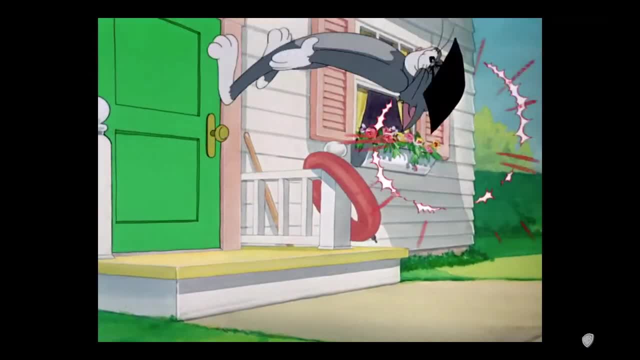 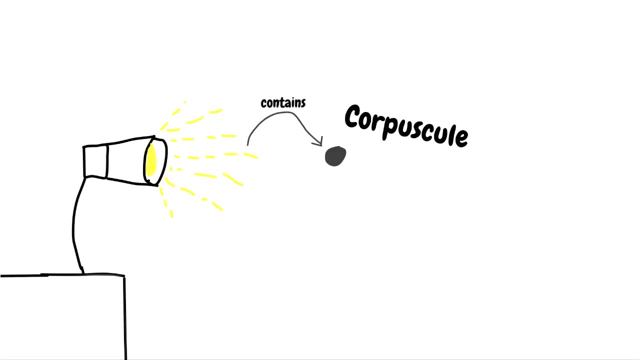 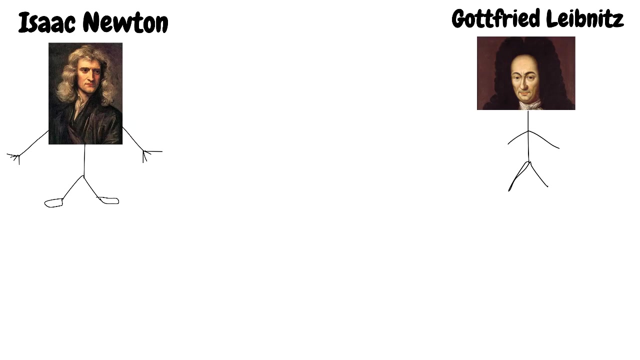 The guy who hypothesized light is made up of particles called carboscules, which allow us to see color when they enter our eyes. Or just the apple guy And Gottfried Leibniz. Both Newton and Leibniz are independently responsible for the foundations of calculus. 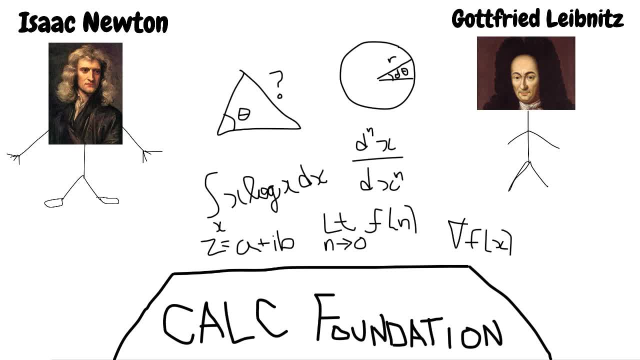 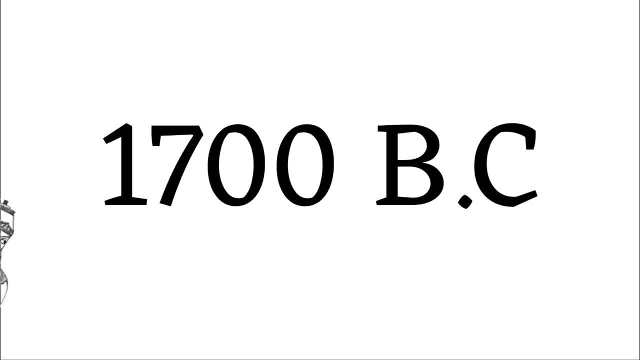 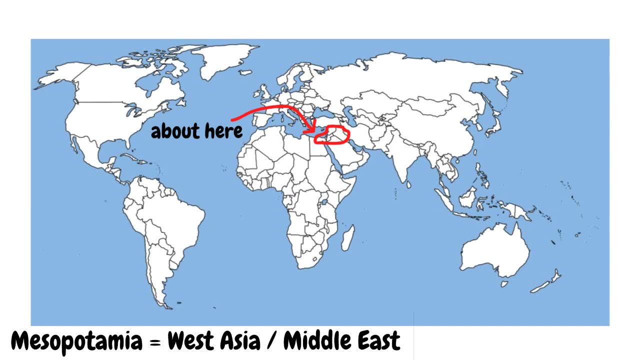 that we see today. Now, if we look at the calculus of calculus, we can see that the calculus starts with them. Of course it didn't. Let's go back in time Too far. Babylonia was an ancient Mesopotamian state comprising of modern Iraq. 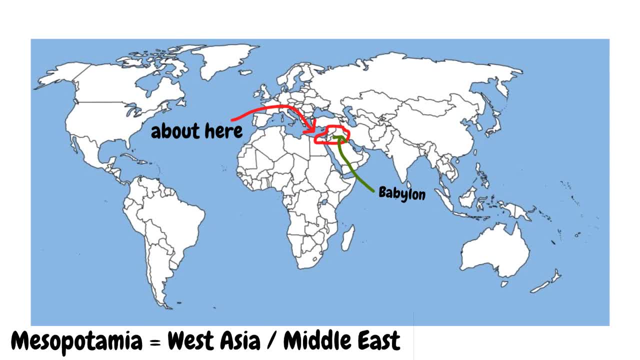 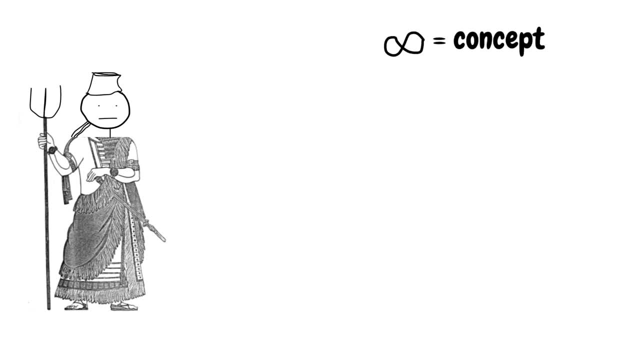 Syria and Egypt. The capital city, Babylon, was about 60 miles from modern Baghdad. Babylonians offered an early intuition on the infinite process. They could determine the square root of a rational number to n Any number of decimal places. A contributing factor was their sexagecimal number system. 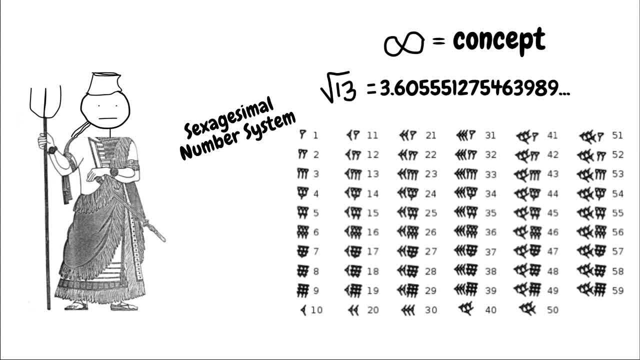 that allowed for a compact notation. Sexagecimal number system has a base 60. That means they represent all real numbers using 60 symbols. This is different from the base 10 or the decimal number system that we use today, The 10 symbols being the digits 0 through 9.. 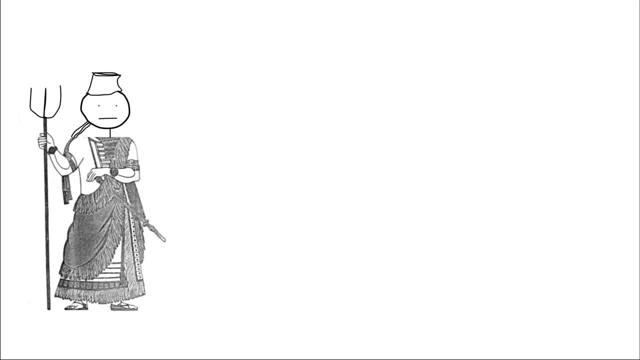 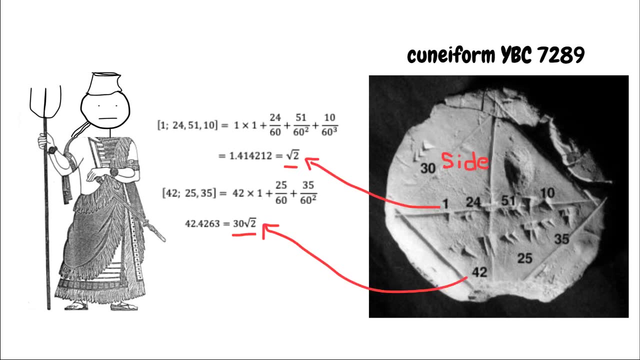 Babylonian mathematics recorded their research and observations on clay tablets called cuneiforms. They were made up of a number of decimal places. They were made up of a number of cuneiforms. This is a famous cuneiform that shows that the diagonal of a square is root 2 times its 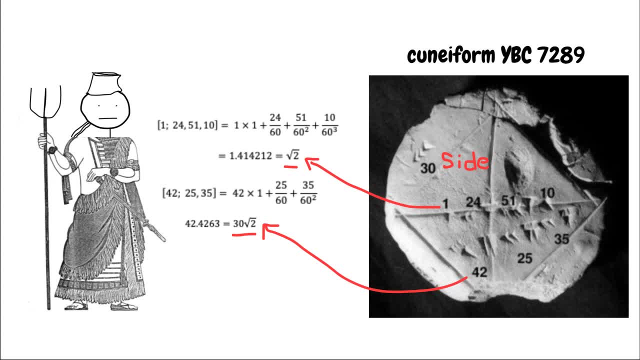 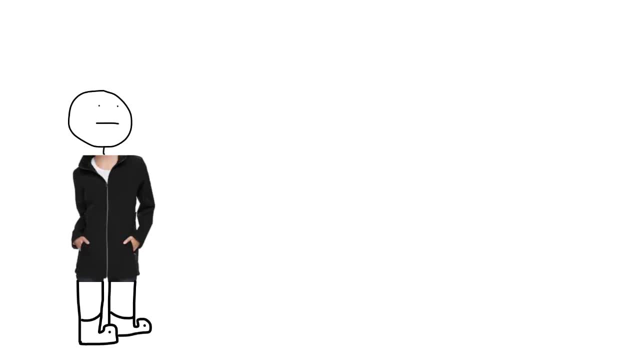 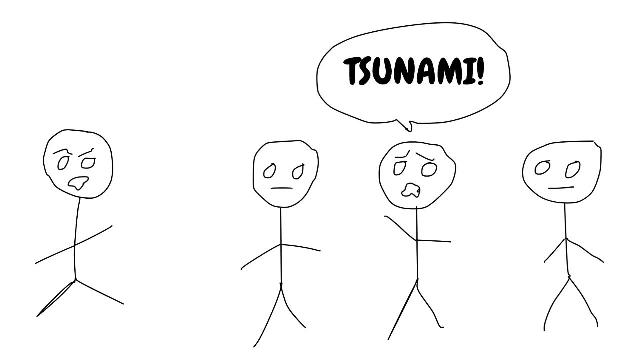 side, They were also able to define other numbers with potentially infinite precision, like the length of the year, or even represent the value of pi. Fast forward to 300 BC, Babylonian astronomers thought everything that happens in this world, from changes in the weather to rise. 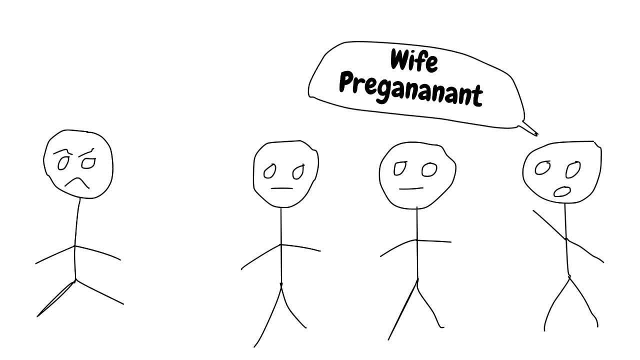 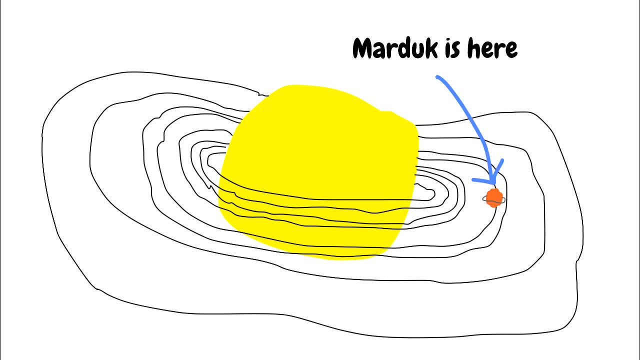 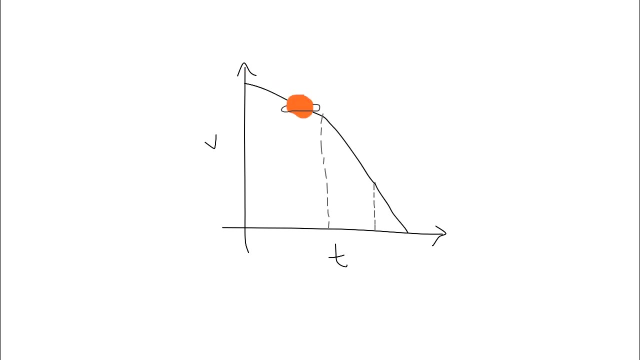 and fall of tides was associated with the motion of planets. So the Babylonians used geometry to study the motion of planets, specifically Jupiter, since their god Marduk was associated with Jupiter. Recording velocities at instantaneous times, they could determine how far the planet travels in an interval of time. This was similar to finding 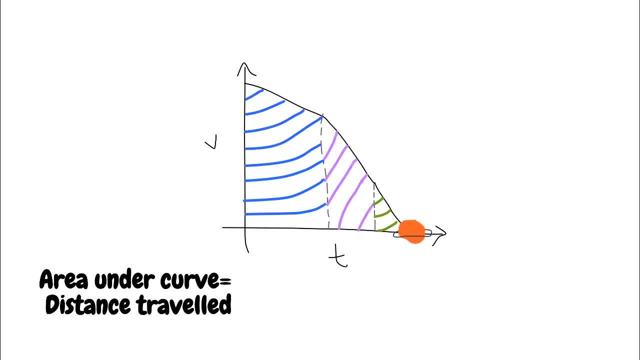 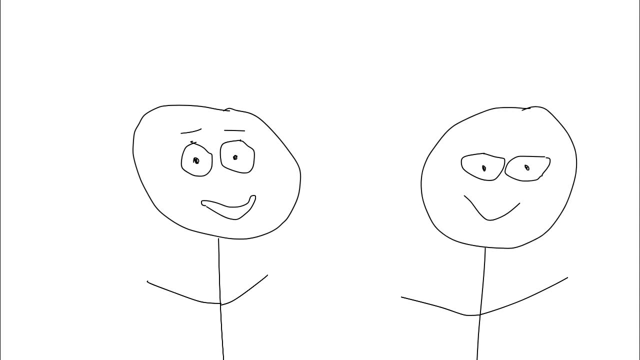 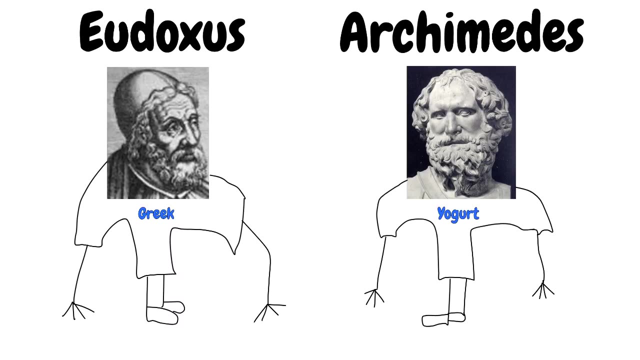 the area under a curve, with the trapezoid rule, which forms the basis of integral calculus that we see today. Did they do everything? Of course, not Around the same time. in ancient Greece were the prominent figures Eudoxus of Nidus and Archimedes. They were able to prove areas of 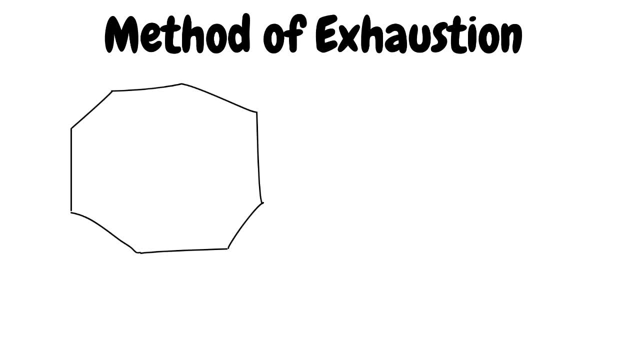 shapes through the method of exhaustion. For neural polygons, say an octagon, we split it up into a number of triangles and find the area of each triangle, then add it up to get the area of polygon. Circles are a special case, since they can't directly be split into triangles. Half a. 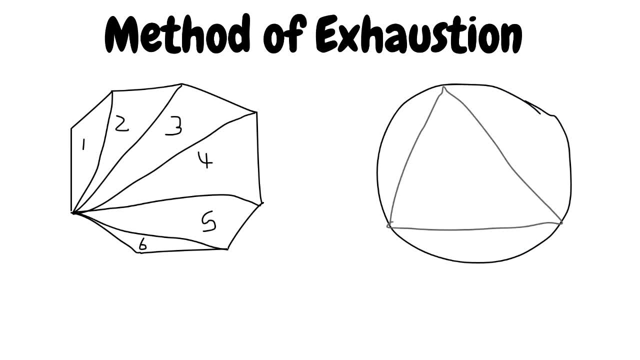 circle is just half a circle. So they inscribed a polygon and gradually increased the number of sides. area of the circle would approximately be equal to the area of the polygon, but the area of the circle would only be the same as the inscribed polygon with infinite sides. 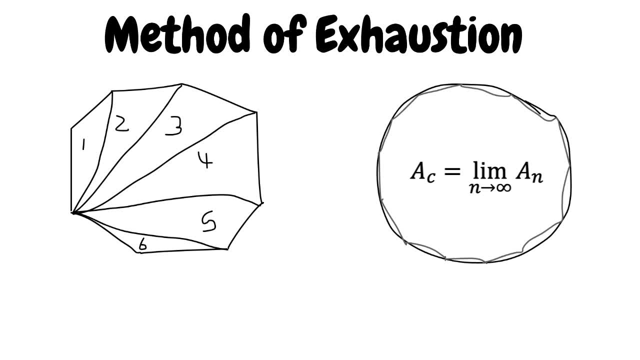 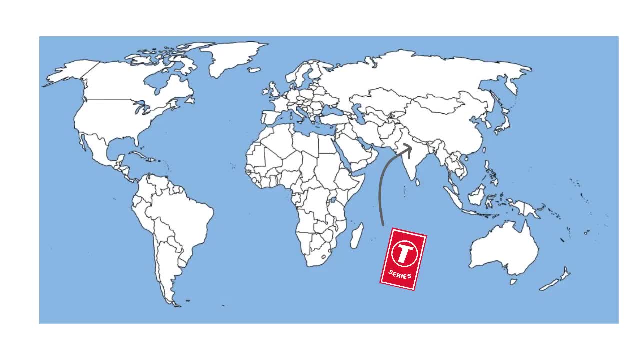 From this we got the concept of limits, and it also incorporated the idea of the infinite process. On to the medieval era. India had their share of contributions too. In the 12th century, mathematician and astronomer Bhaskara II wrote the Siddhanta Shadomani. 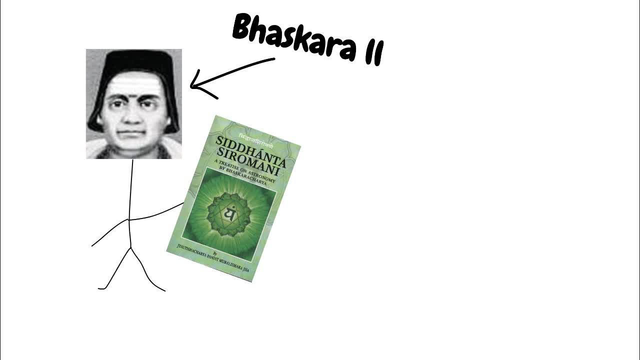 which contained texts in astronomy with proofs. using calculus, He proved that, at its highest point, the instantaneous speed of a planet is zero. Actually, I don't know what that means, but that's what it literally says in this paragraph of a news article in a language you don't care about. 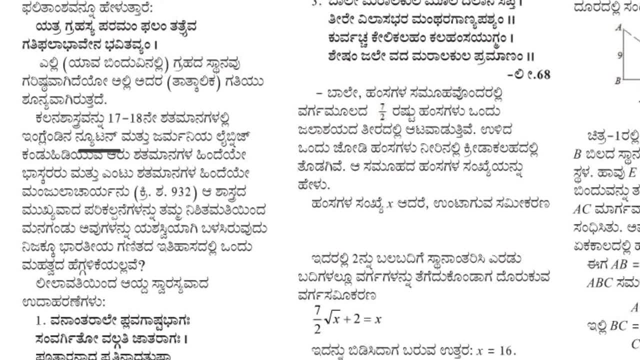 And this paragraph talks about how some English mathematicians called Newton and Leibniz are known for this discovery, even though Bhaskara said it a few centuries earlier. But we're not done with the theory. One of the greatest mathematicians and astronomers in the 14th century India. 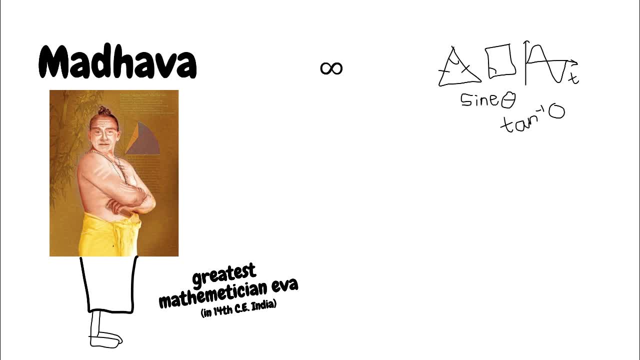 Madhava linked the idea of infinite series with geometry and trigonometry. He was able to formulate infinite series expansions for sine cosine, arc, tang and even pi. So you see these expansions here, You know the ones we call the power series expansions. 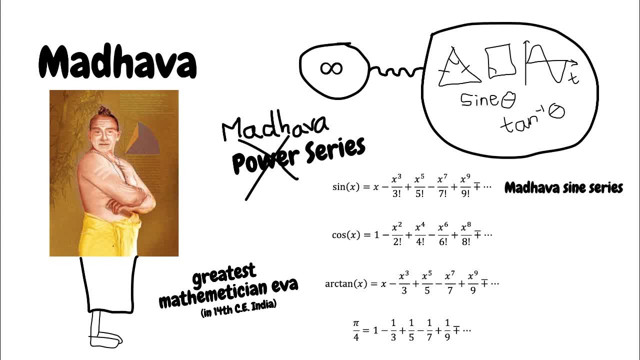 But nope, they're called the Madhava series, This is the Madhava sine series, this is the Madhava cosine series and this is the Madhava arc tangent series. But if he did figure out that they are infinite, then why did he say infinite series in the end?